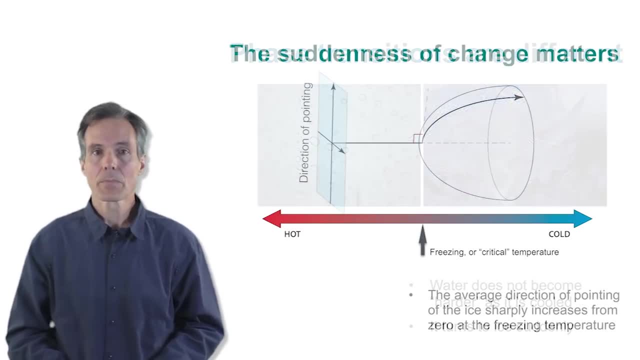 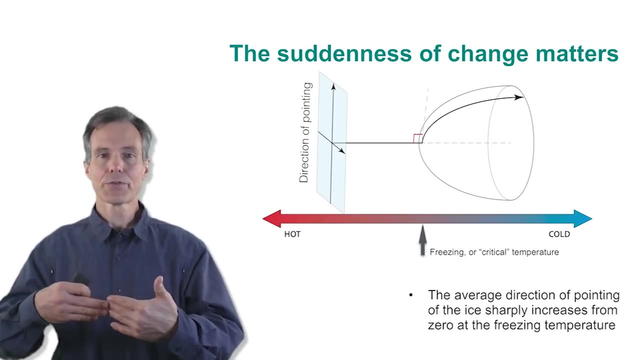 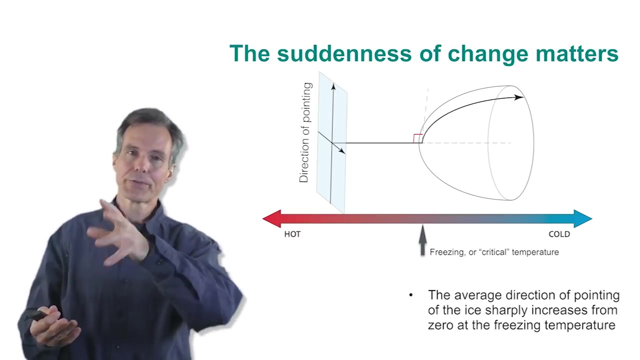 that suddenness of the change matters. If we think about the ice crystal, it has a direction of pointing And that direction of pointing comes into existence sharply as we lower temperature through the freezing temperature. In the diagram, the circle indicates the directions in which the ice crystal could point. The line is the state of water, where 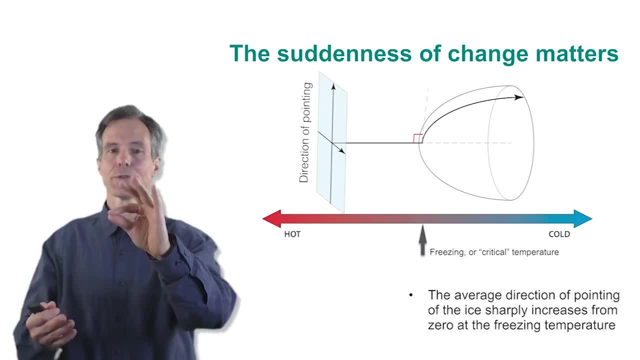 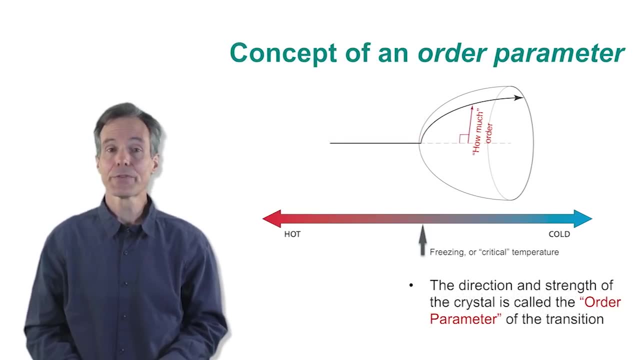 there is no direction, And the freezing transition is one where suddenly the ice points in a particular direction. The direction and strength of the crystal are what we call the order parameter of the phase transition. They give a sense of what kind and how much order it has. The order. 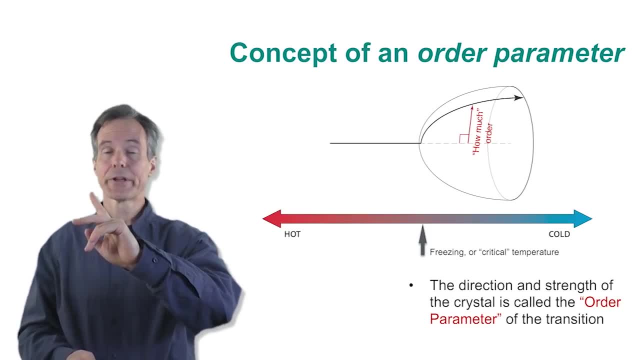 parameter has two properties: One is a direction, which is arbitrary, and the other is a strength, which has to do with how far we are below the freezing temperature, And this gives an idea of how globally the ice crystals are lined up and how rigidly they're in that configuration. 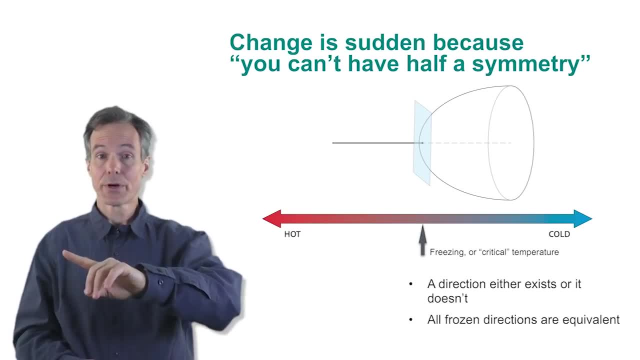 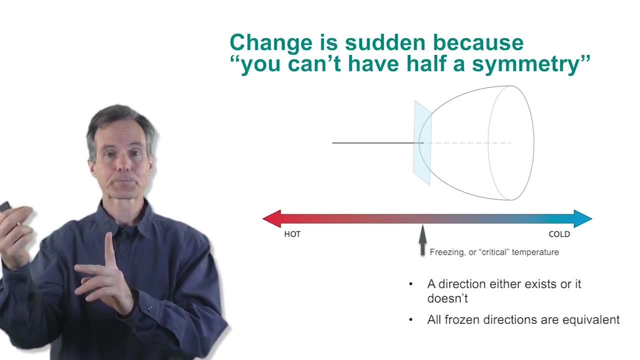 If you talk about a direction, you either have one or you don't. You can't have half of a direction. If we want to understand the reason for the suddenness with which the order parameter comes into existence, we introduce the important concept of symmetry in phase transitions. 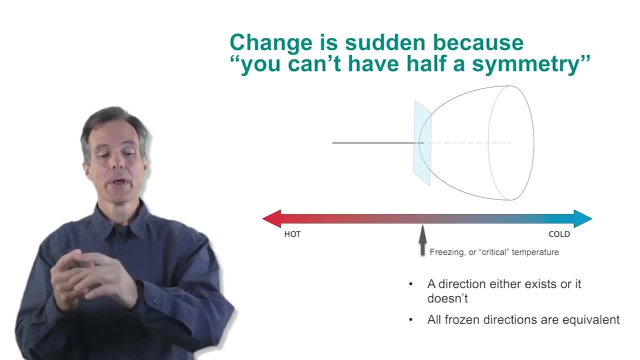 For a frozen state, a direction either exists or it doesn't. The underlying water is symmetric, and so any frozen direction is equivalent to any other, and yet, in order to freeze, you must choose one, Because you can't have half a symmetry, you can't be an equal mixture of frozen and many. 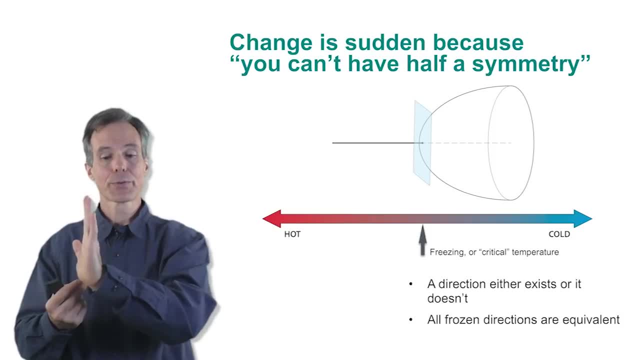 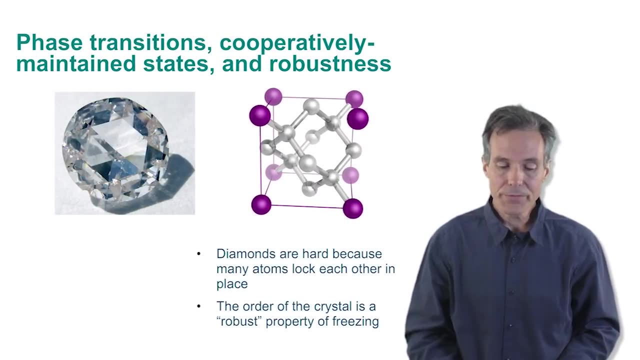 directions, and it's that requirement to choose that creates the suddenness in the blue panel with which the order parameter sets in. This causes phase transitions to play a very important role in our material world. They actually are responsible for most of the robust patterns we see, and it's through something. 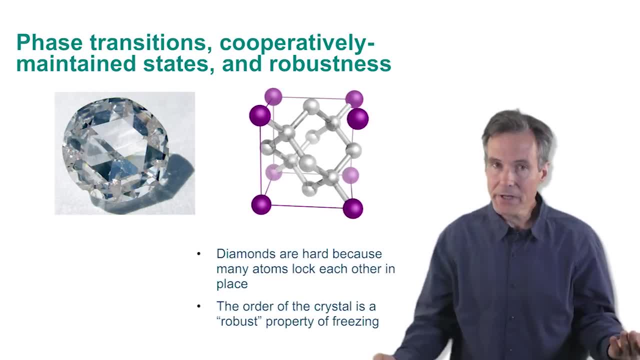 that we can call cooperatively maintained states. Everybody knows the expression, the expression diamonds are forever, which is a statement that they're so hard they'll outlast almost anything, But any given atom in a diamond is very easy to move. Why then, 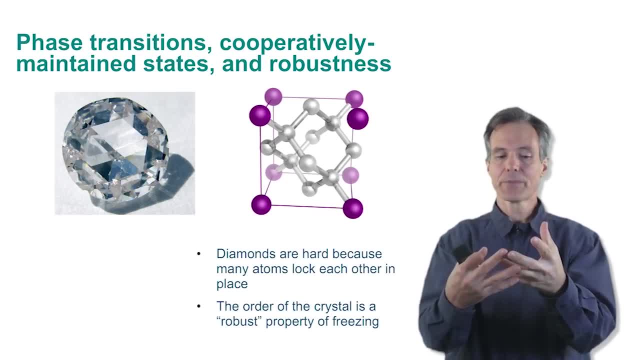 would a diamond be hard. It's hard because all of the atoms in a macroscopic scale interlock with one another in a crystal structure and you can't move any one atom without moving all of the others. The order of the crystal is the robust property brought into existence. 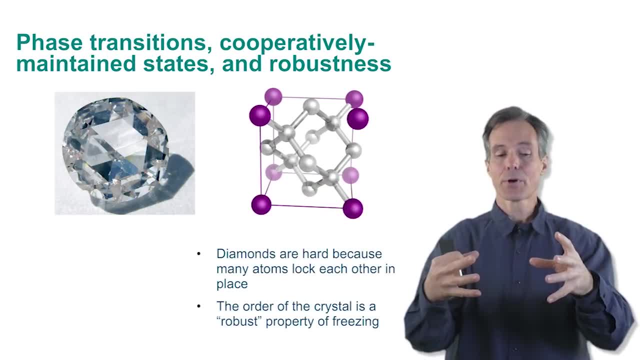 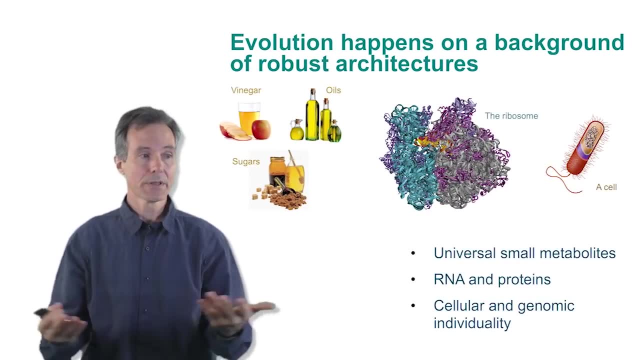 if a carbon gas freezes to a diamond, And that is the property made robust by the phase transition itself. Now evolution in the biological world happens in a background of robust architectures. There's a variety of small molecules, like acids such as vinegar, or oils or sugars, that play universal 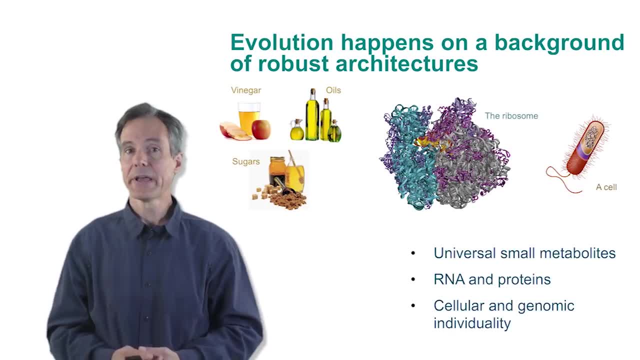 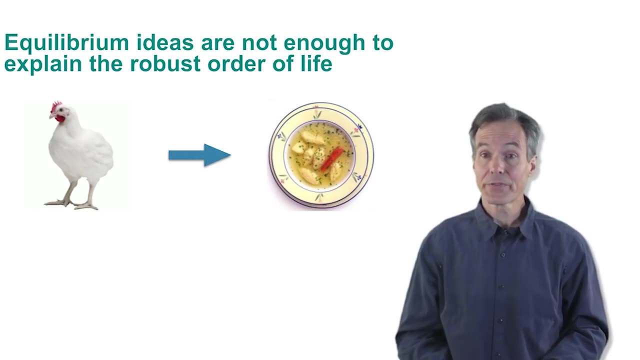 roles in all living things. There are larger molecules like RNA that make up the ribosome. There are architectures like cellularization. All of these are universals within which evolutionary dynamics interact. But equilibrium ideas are not enough to understand the nature of living, robustness or the cause. 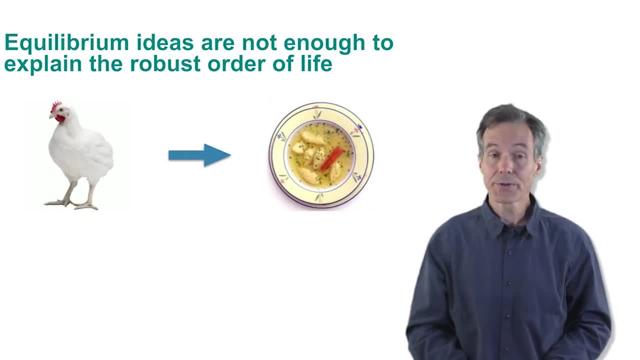 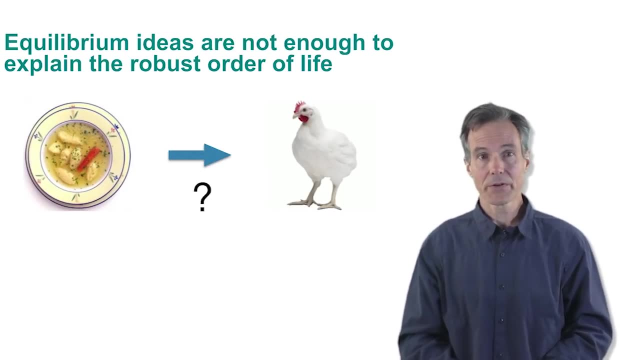 of it. So consider: if I begin with a chicken, I can turn the chicken into chicken soup. But if I start with chicken soup, even though it has the same ingredients, no one has understood how to recreate a chicken from that. A classic example is Stanley Miller's 1953 experiment. 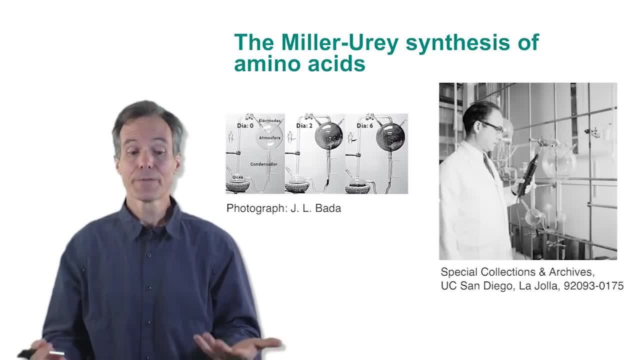 that made the study of the origin of life a serious scientific topic for the first time in history. Miller took a variety of gases, excited them with an electric spark and saw that over a period of time, the transparent mixture of gases was converted to a variety of darker 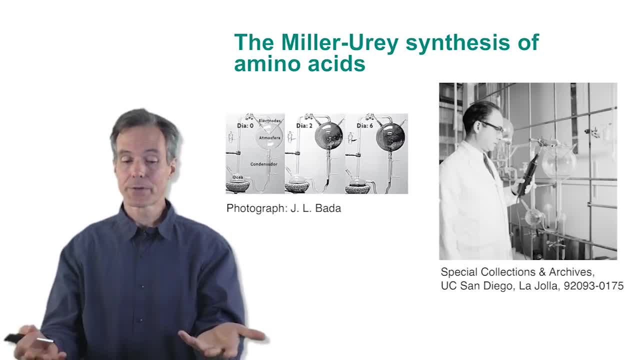 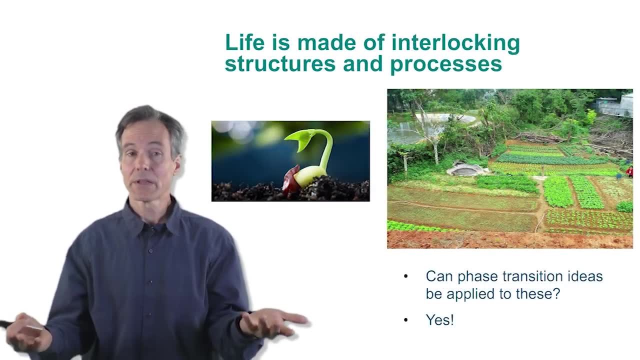 and darker tars, which contained amino acids, which are the materials of which living systems are made. But these amino acids were not life, just like the chicken soup is not the chicken. Of course we understand why: because life is made of interlocking structures and processes. 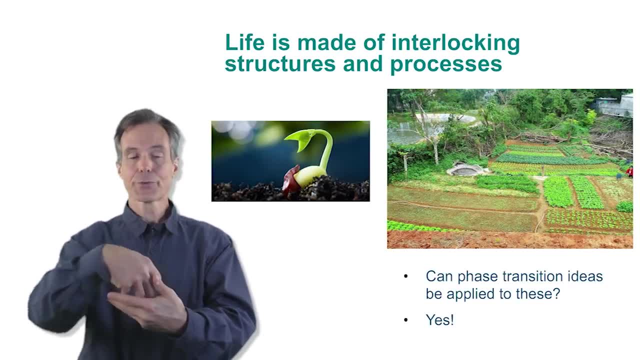 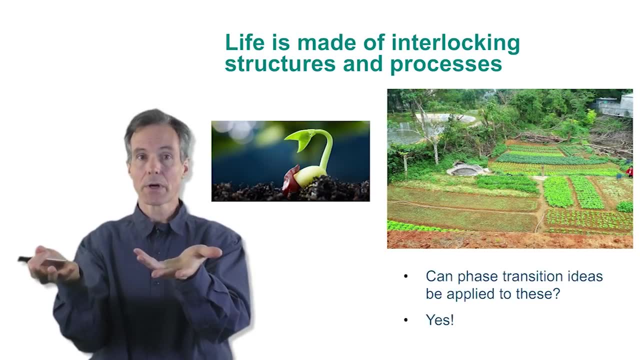 If you think about a seed germinating, this structure is being built. but when the structure is built and a field becomes green, all of these leaves do the work that make it possible to build the structure in the first place. So we can ask if we understand robustness and its relation to phase transitions and equilibrium. 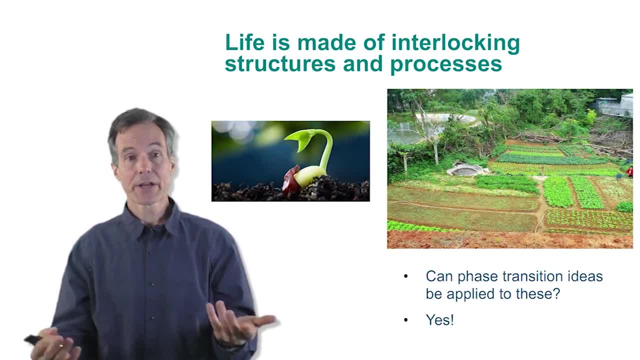 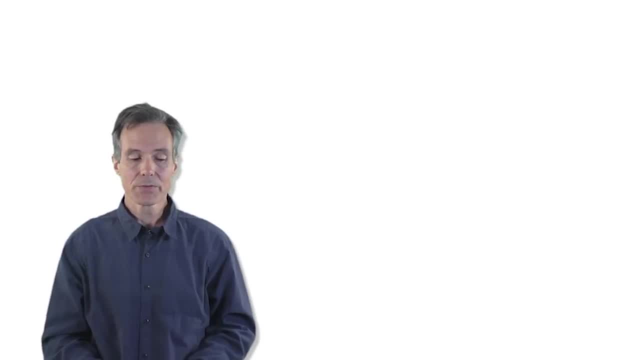 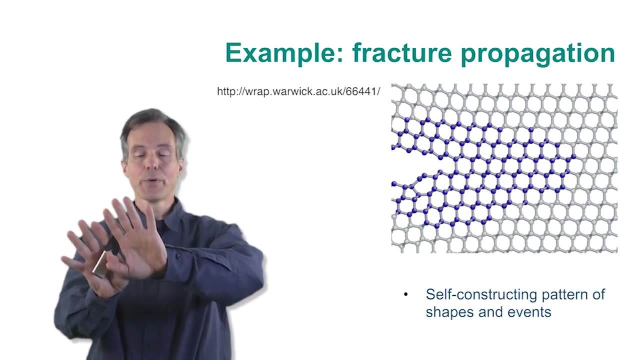 can the same ideas be applied to a dynamical interaction of structures and processes? And in fact they can. Maybe the easiest system in which to understand this directly from a picture is the example of fracture propagation. We begin with a lattice of atoms bonded together and we stress it in some way so that, to relieve the stress, it might separate. 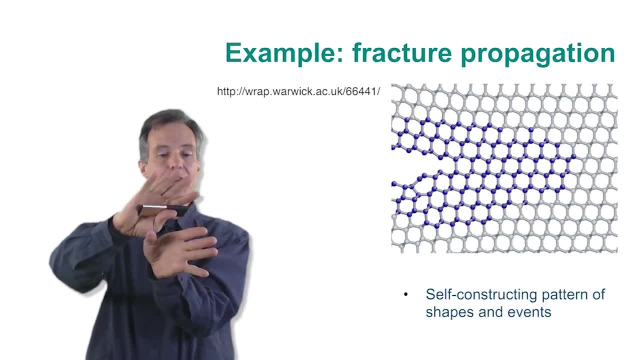 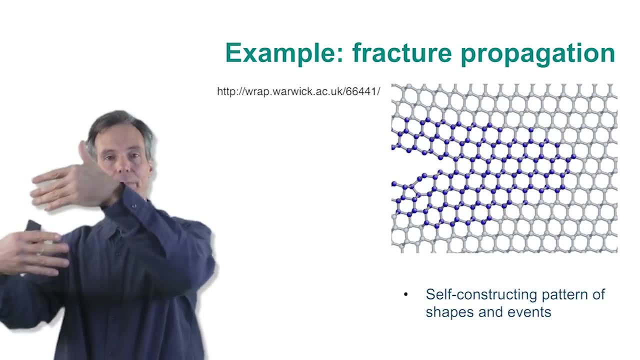 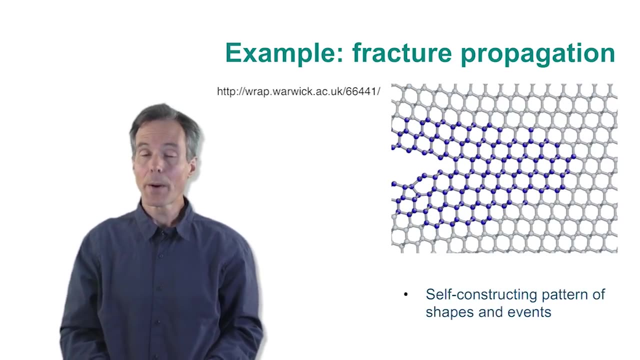 If we put a nick in that system, we can watch the fracture grow. It's the propagation of a self-reproducing pattern of bond breakage and realignment of the stress field shown in purple in the surrounding bond. The sense in which fracture propagation is a cooperative effect is that the breaking of bonds occurs at the scale of single atomic diameters. 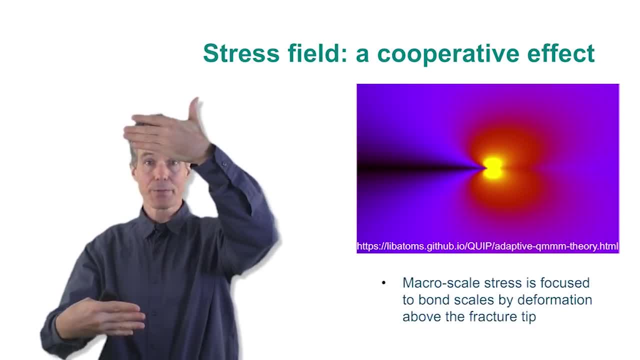 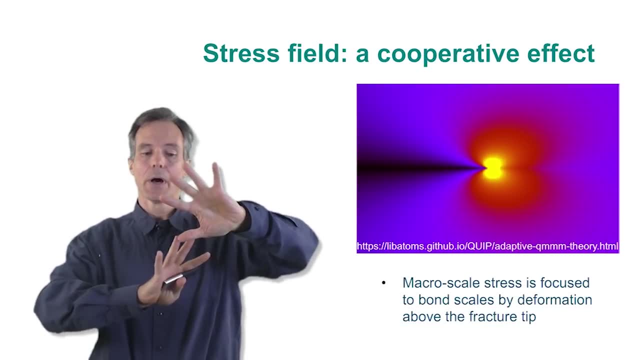 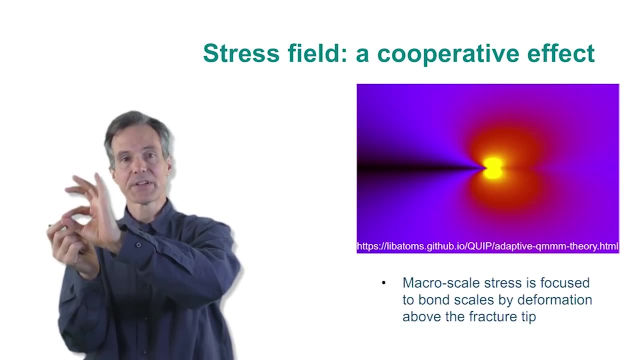 but the stress field is uniformly distributed throughout the entire material. The macro-deformation from the part that's already ruptured allows a weak energy density distributed throughout the material to focus as the bright light shows you all the way down to a single bond diameter. 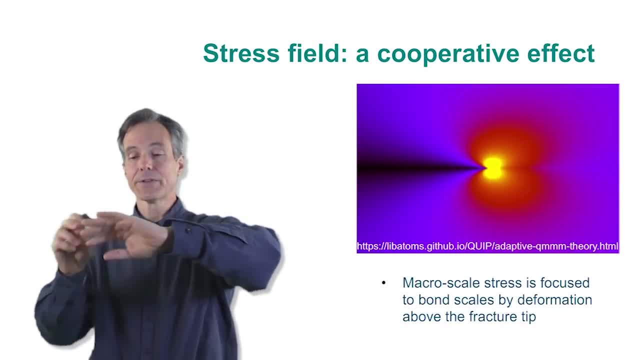 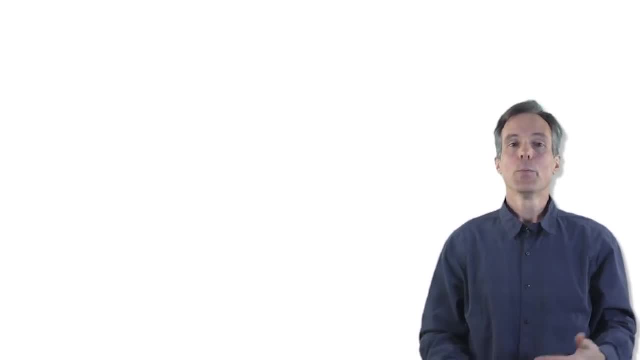 And it's that focus that causes the stress field and the structure to break And the bond breakage to repeat and propagate as a self-reproducing pattern. We can understand the spacetime patterns that are formed in these kinds of transitions as states of order. 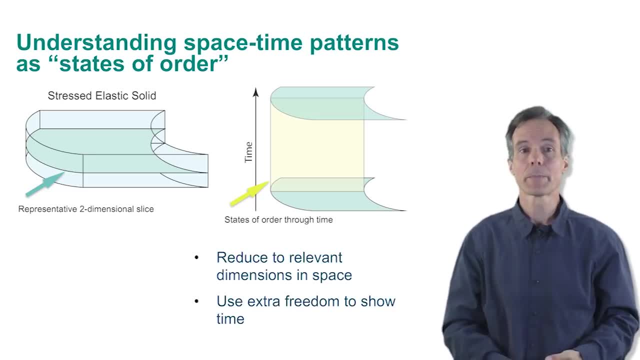 the same way as we can understand a crystal orientation as a state of order. One way to do this is with diagrams. Suppose I took a stressed elastic solid which is a block, and I turn it so that it's bent. I don't need all three dimensions of that, so let's take a slice through it that represents the important effect of the bending. 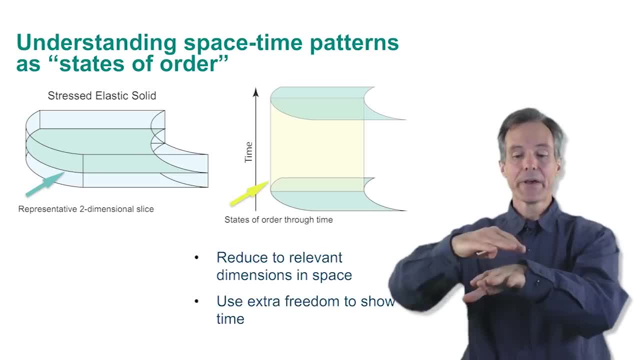 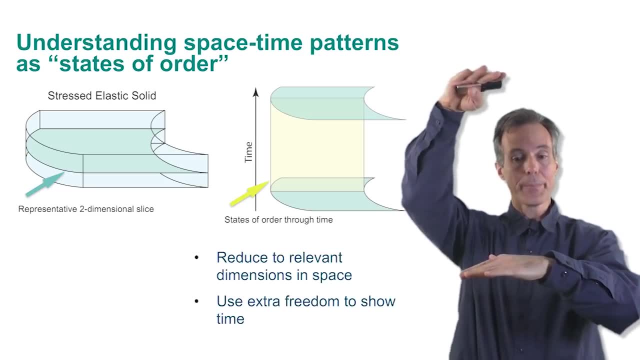 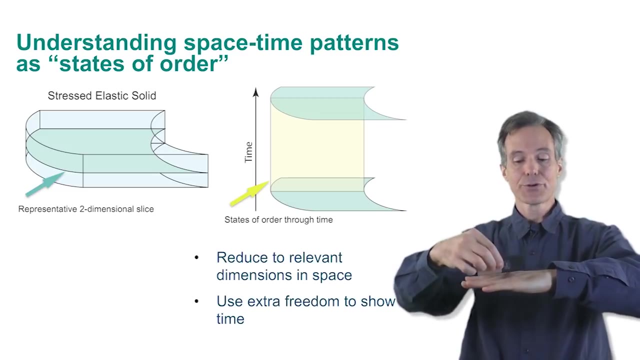 and we'll draw that green slice on a plane. Now I have an extra dimension and I can use time to represent the extra dimension the same way as if I stacked sheets of movie film up to make a stack And then I can look at the pattern of a particular part of the material through time as a yellow sheet. 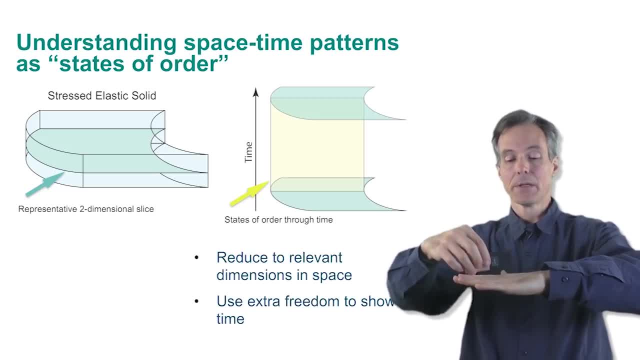 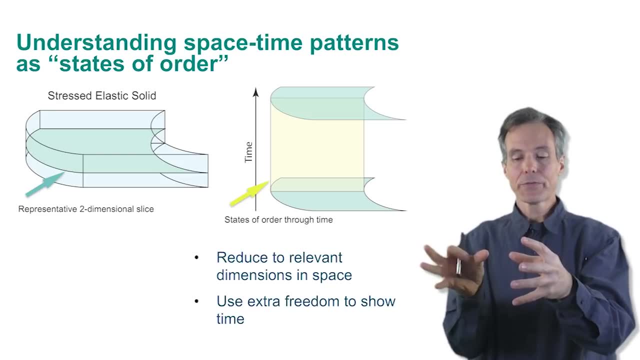 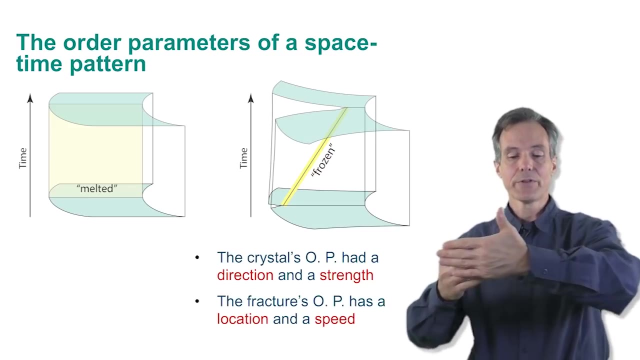 and I can ask what patterns are displayed in that spacetime diagram? In this way we can compare the stressed material without a frame and we can see that the stress field is the same as the fracture, which is like a kind of melted state which has all of its symmetry. 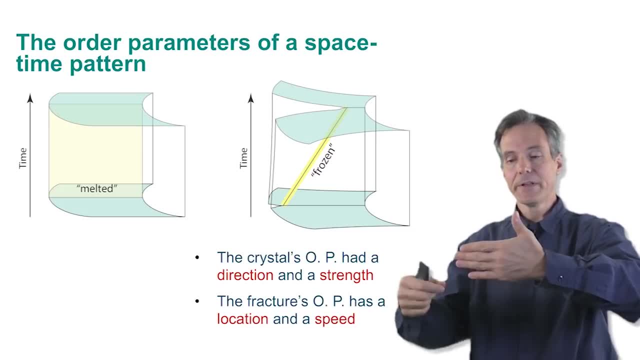 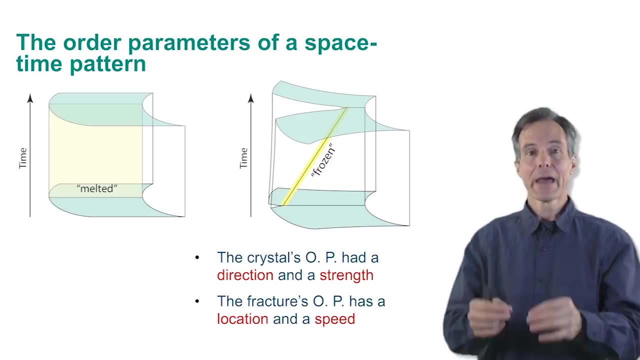 Here you have a uniform but dilute stress field that simply persists through time If a nick is introduced and the fracture propagates. we see this in a space diagram as illustrated with the yellow line as this pattern of a stress field and the fracture tip. 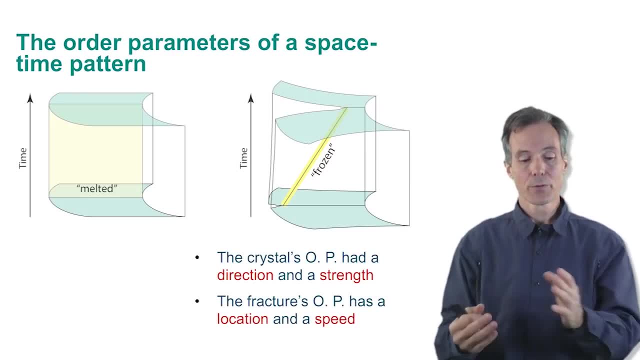 which move in a uniform way through space and time. Now remember that we said for the crystal: the order parameter has two properties. The other is a magnitude which follows from the laws of the underlying physics. The fracture has something like that in time. 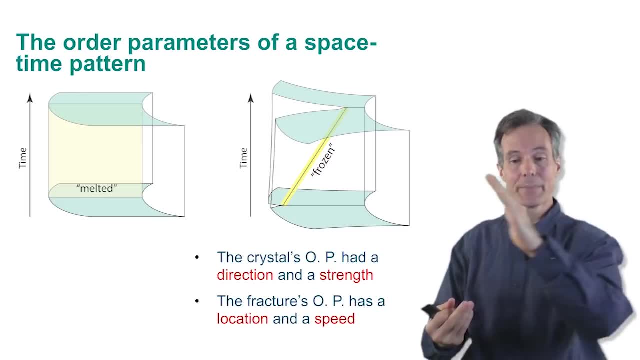 Its position relative to an arbitrary origin of time can be anywhere, because this is a direction of symmetry, But the speed at which it moves is determined by the underlying physics, and that's a property that you can predict, like the hardness of a crystal. So we see that the concept of phase transition and the spontaneous creation of order 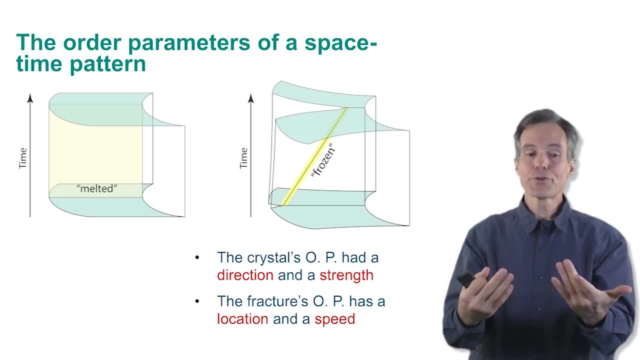 exists in the dynamical realm. Frozen motion doesn't mean motion that's caught and that stops. That would be the end of motion. Rather, frozen motion is motion that's made robust by cooperative effects in phase transition. What might be the order parameters of life if we try to use dynamical phase transition? 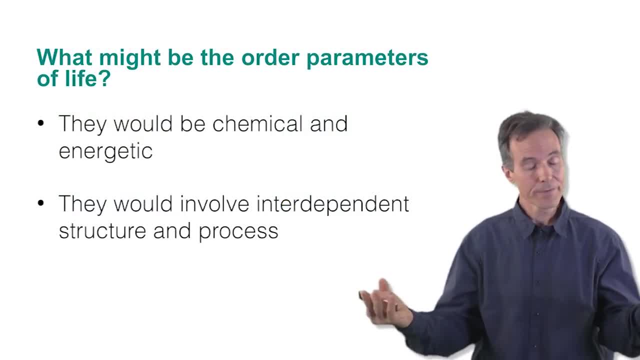 to understand the robust, universal things that it's built of. Well, first we know they would be chemical and energetic, because life is an energetic process living in a chemical medium. We also expect that they would involve interdependent structure and process, where the structure carries the process and the process builds the structure. 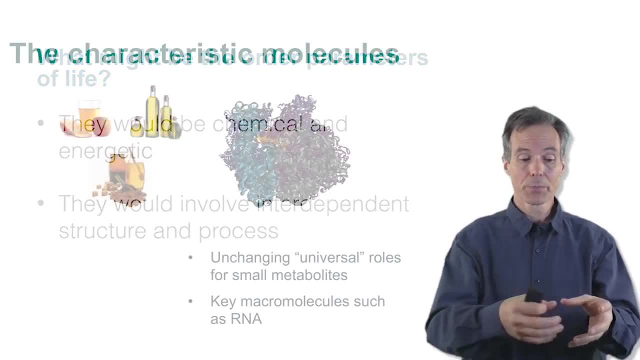 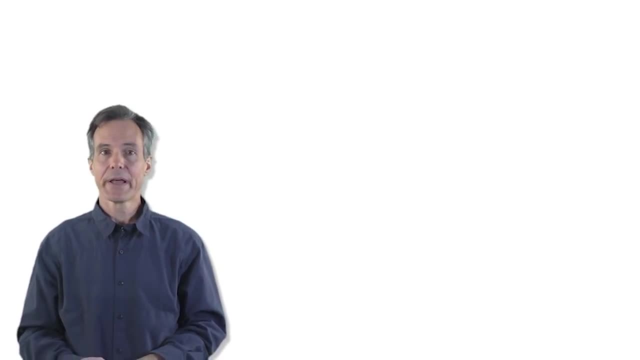 Some candidates for these would be the characteristic molecules, the small metabolites that play the same roles, or the RNA. But another property could be found at the scale of the entire planet, and this is the effect that our biosphere has on the great biogeochemical cycles. 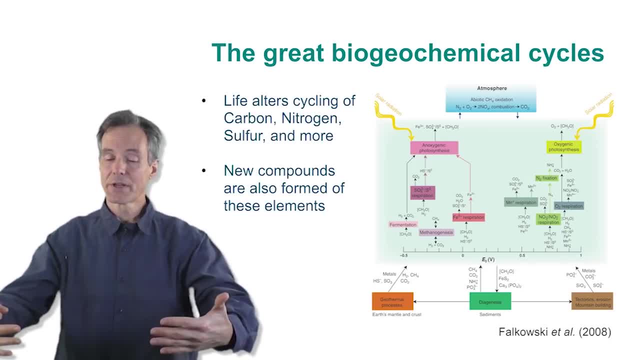 The presence of living systems alters the cycling of carbon nitrogen, sulfur and many more elements, as well as water In the process, or the way that it makes that motion possible is by building new compounds out of these elements, which would not exist in a planet that did not have a biosphere. 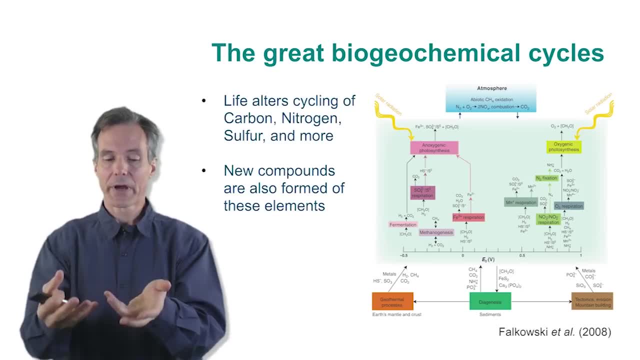 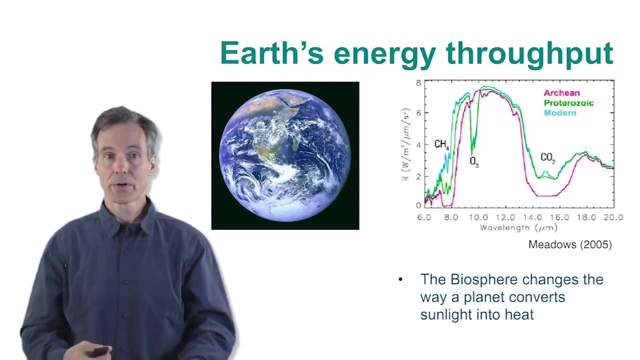 And the regular patterns in these changes are eligible to be the order parameters for life as a phenomenon on a planet. Another possibility would be Earth's energy throughput as an entire system. Earth is a green planet. There is no other green planet. for the same reason, in our solar system. 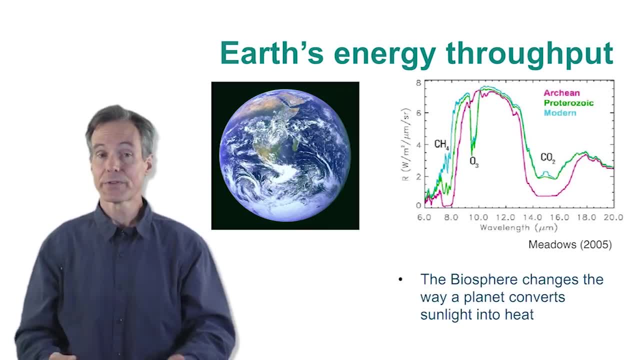 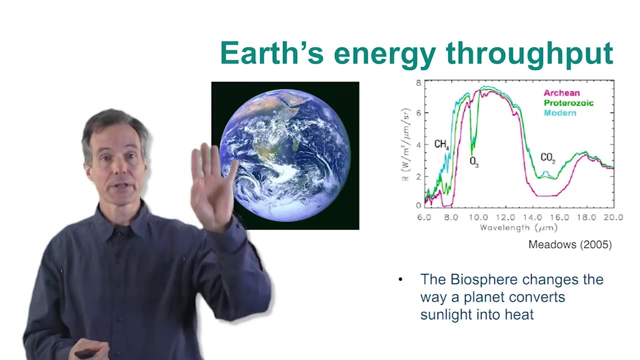 and that's because the biosphere and its pigments have been brought into existence on that planet. The biosphere has also changed the composition of our atmosphere. In particular, it's brought molecular oxygen into existence in the atmosphere, which could be seen from space as sunlight shines through. 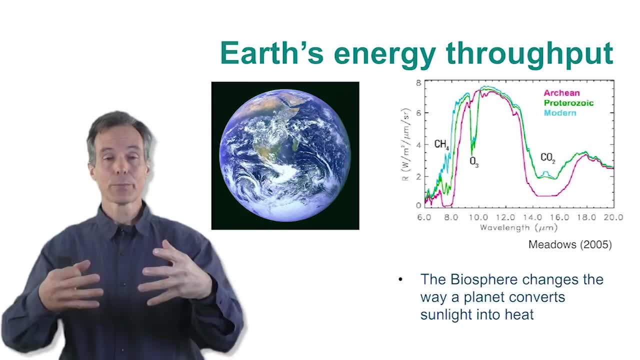 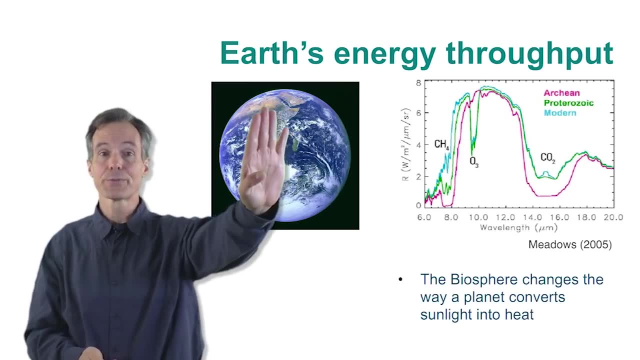 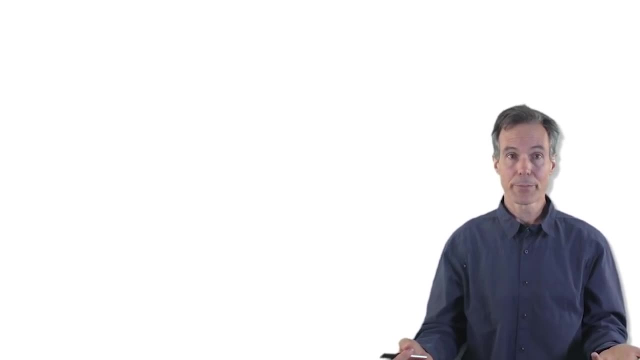 And the study of the way living systems change. atmospheric composition is one of the ways scientists can do that. Scientists look for the possibility of life on planets that are too far away to allow us to see anything else. Another possible characteristic of life that could be an order parameter. 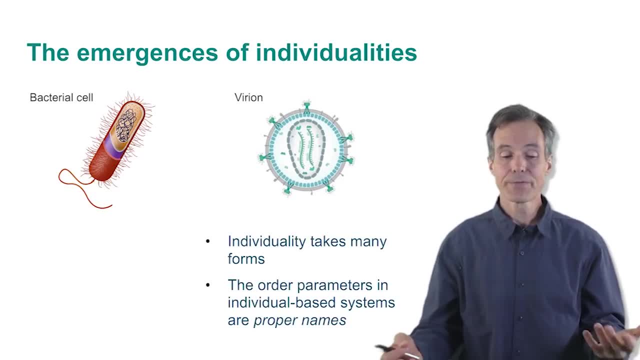 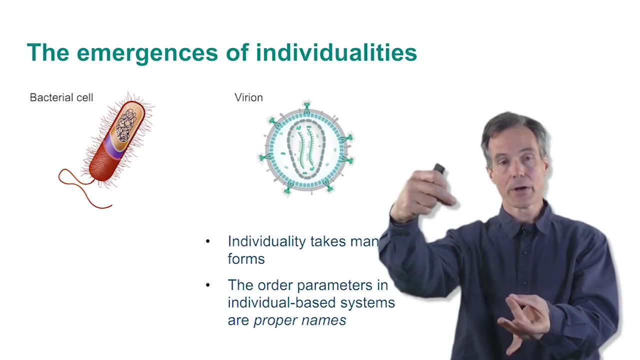 is the concept of individuality, which has emerged in many different ways. A bacterial cell is contained in space and has a protected environment, but it also has a molecular genome. A virion has the genome, but not with the same connection to energy and metabolism. 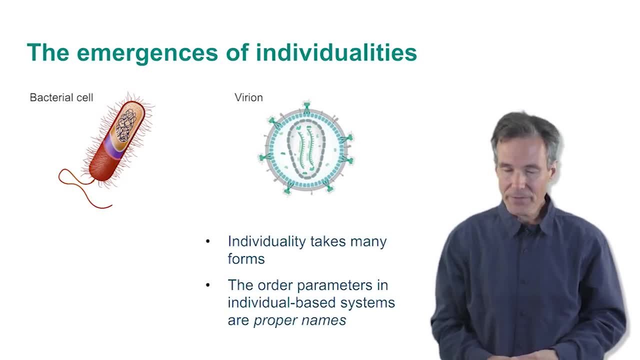 So we see that individuality takes many different forms. Life is fascinating in this regard because all of the phase transitions I told you about before now have an order parameter that takes one value throughout the bulk. But if we want to understand the kind of order that comes into existence with individuality, 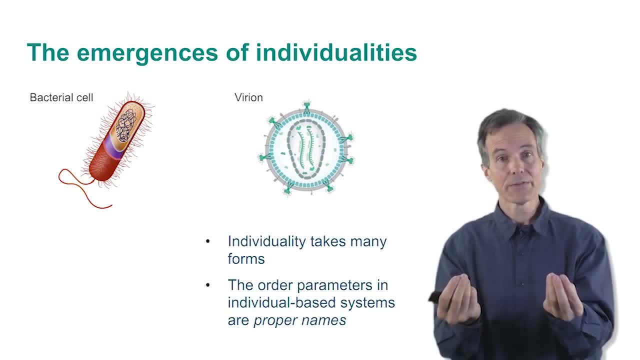 we encounter something fascinating that we normally discuss in the humanities, which is the need for proper names: Harry, Jane and June. So we can think of individuality as the phase transition whose order parameters are proper names. So the take-home messages from this lecture are first: 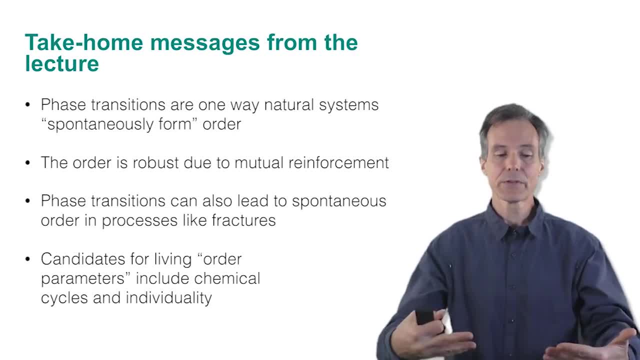 that phase transitions are an important way that natural systems spontaneously form order that's not imposed by their boundary conditions. The order is robust because the components mutually reinforce each other and make it difficult to change locally. We know that phase transitions can also lead to spontaneous order. 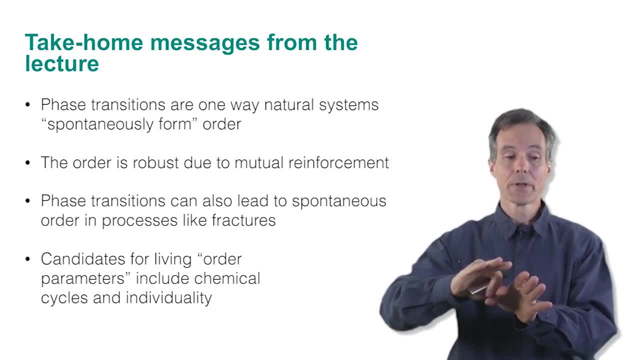 and we can see the example of fracture propagation as an instance of how this works. And it's important to say that we don't know how much of the order of life can be understood through this concept of dynamical phase transition, but candidates for order parameters of these phase transitions might include